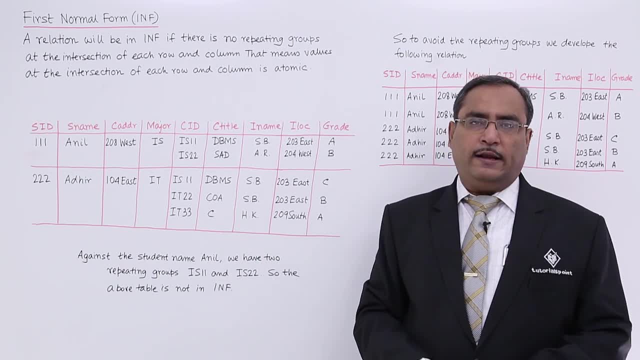 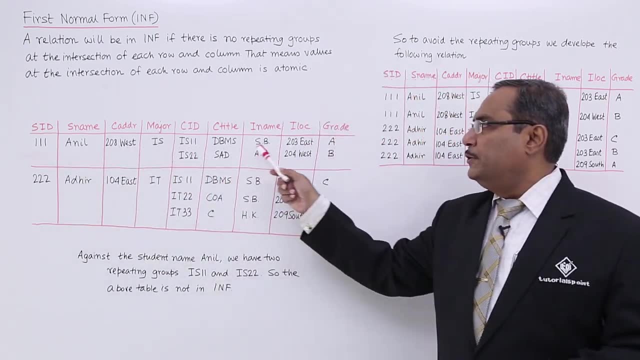 Now this is a table which is not in 1NF. The questions might be asked, why? Just see, if you consider this particular column and if you consider this very row, then at the intersection you are getting non-atomic data. 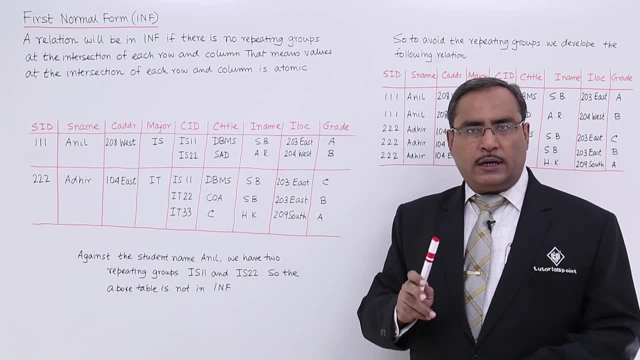 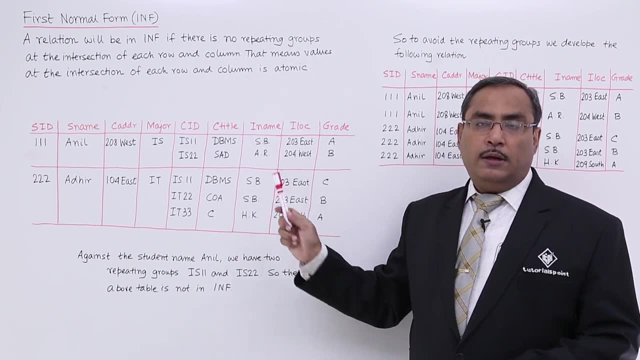 That means that is one data, that is another data. So two data are residing in the same cell at the intersection of one row and column. So that is why they are non-atomic. But 1NF says that all the data items at the intersection 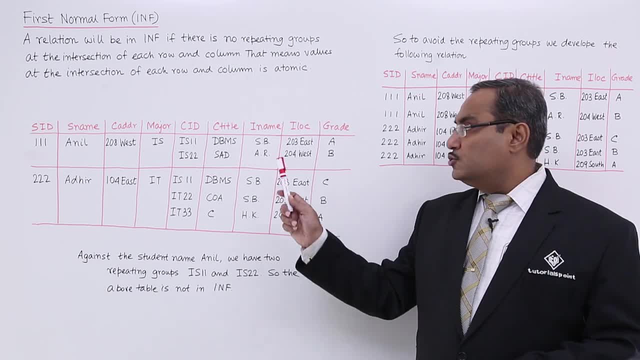 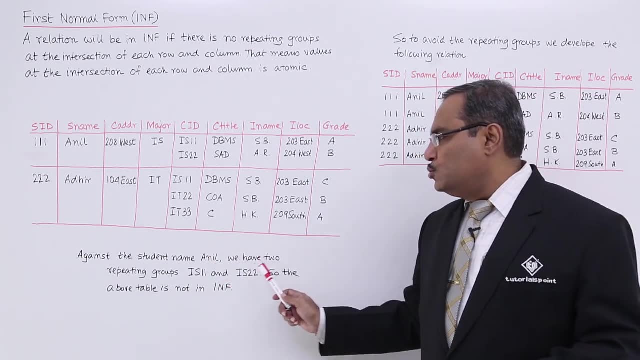 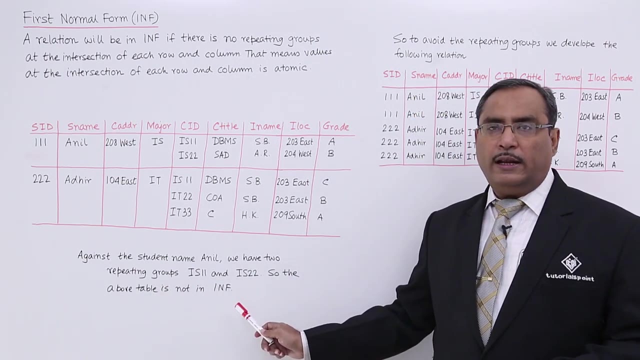 Of each row and columns must be atomic in nature. So that is why it is non-atomic. Another thing is that against the student name, say anil, we have two repeating groups: IS11 and IS22.. So the above table is not in 1NF. 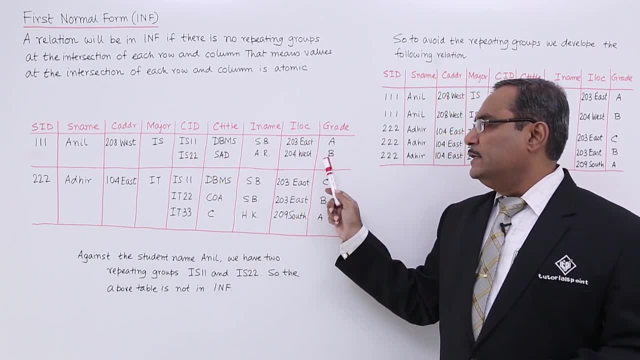 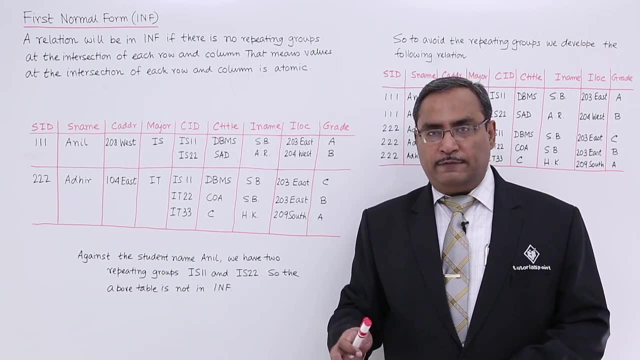 So for the anil I am getting two repeating groups are there and these groups are there, So repeating groups are occurring. So that is why we are getting this one as not in 1NF. So if I want to call it 1NF, 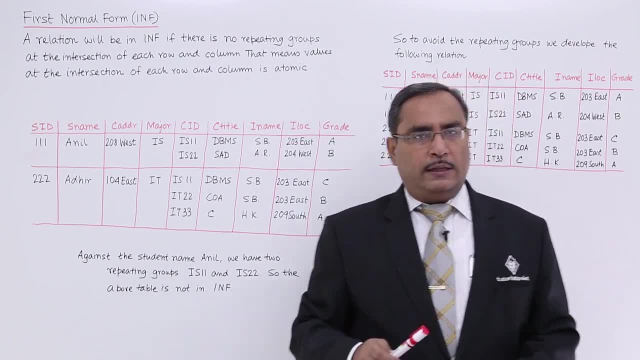 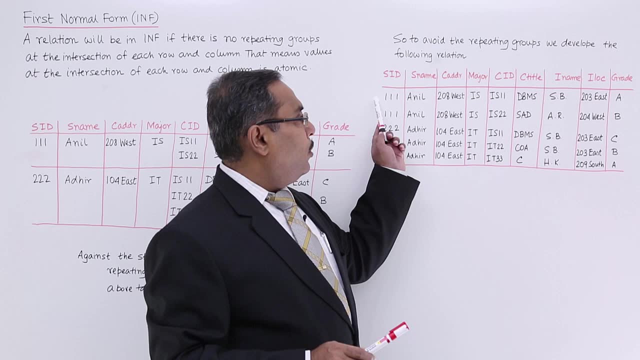 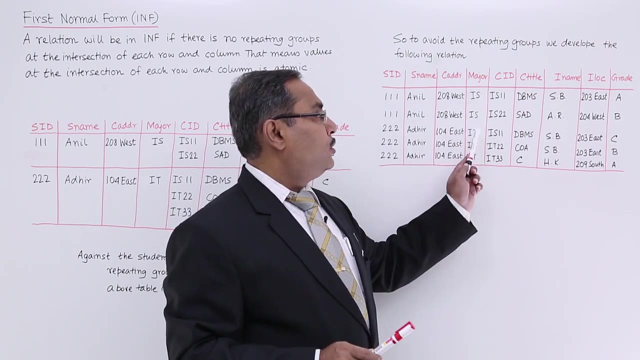 I want to bring this particular table to the 1NF. then the respective relation will look like this. So here you see. O'Neill had two courses, So the O'Neill details has been written twice. Othid had three courses under the major IT. So Othid record- Othid information. 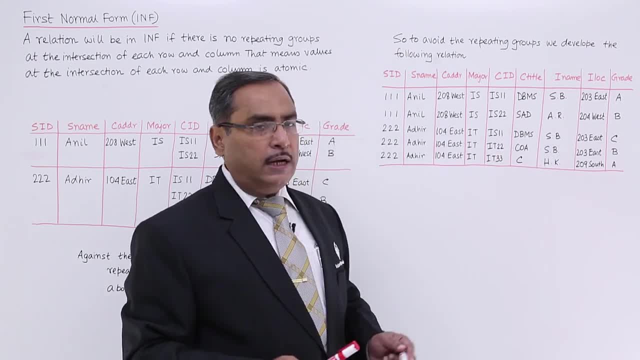 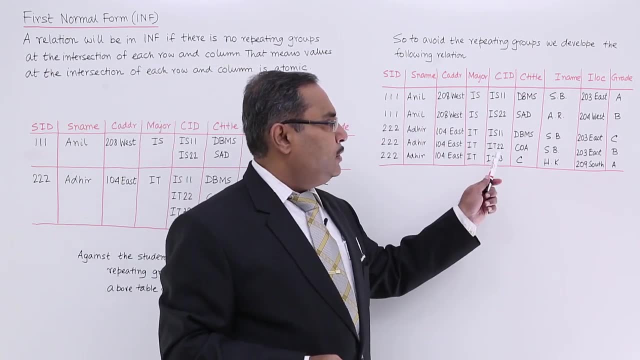 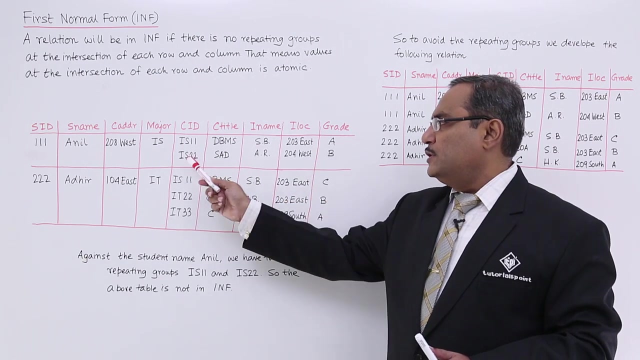 has got repeated thrice And in this way the table does, the relation does. obtained is in 1NF. Here you see, at the intersection of each row and column you are getting atomic data And there is nothing like this. repeating groups type of that means one bunch of information. 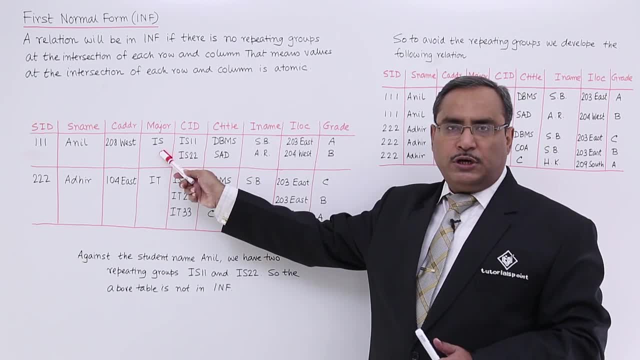 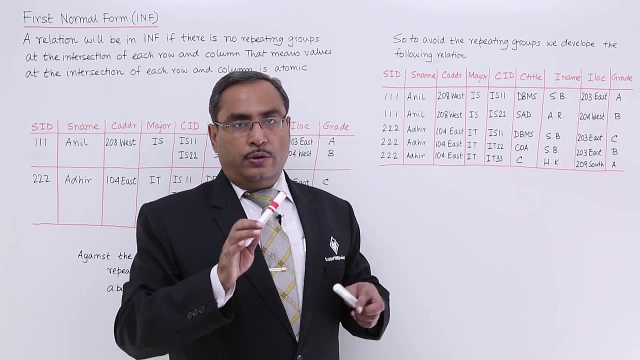 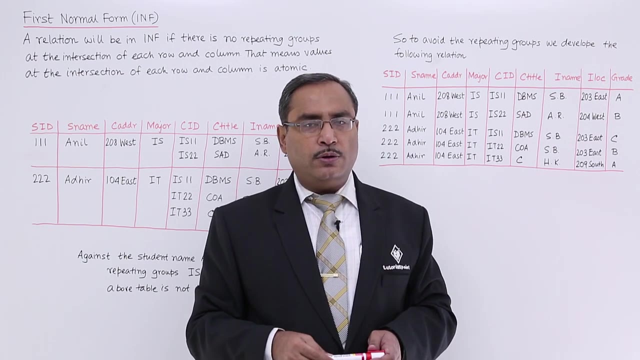 another bunch of information for this- against one major value, that is, IS. So it was not in 1NF, but this relation is in 1NF. So here we have discussed, with some example that what is 1NF or first number form. Please watch the next video. 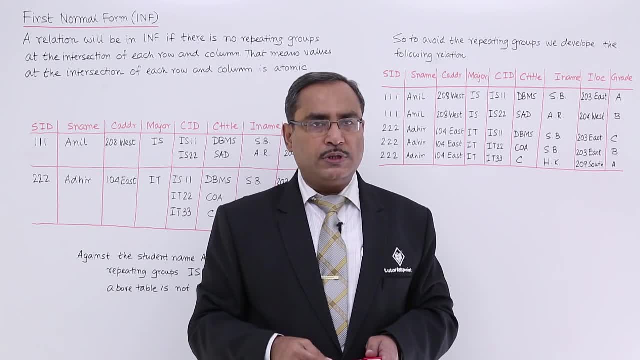 There, we will be going for 2NF and other normal forms. Thanks for watching this video.